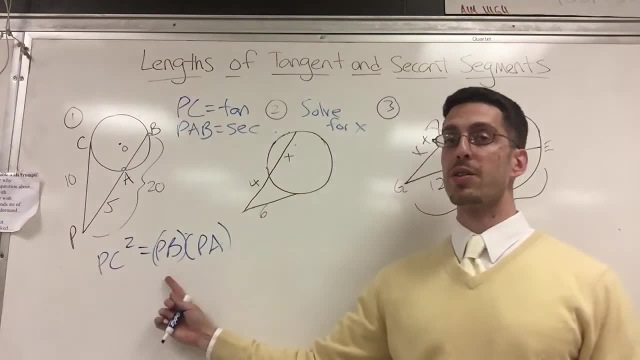 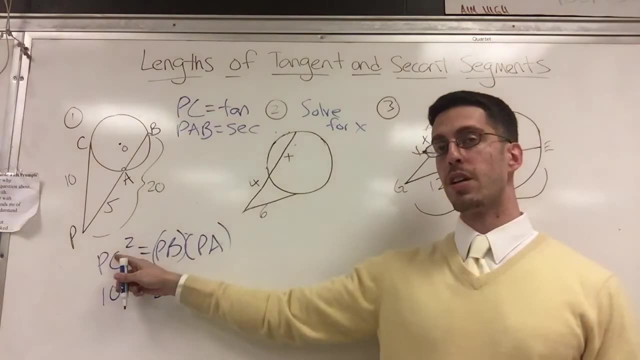 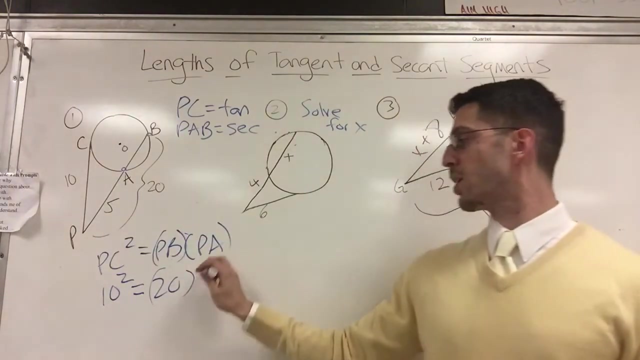 the concept: Tangent squared equals entire secant times external secant. Let's look at numbers: 10 squared equals what? 20 is the entire thing times the outside, which is 5.. Obviously not drawn to scale. I don't have a scale, Didn't use it. Okay, let's see: 100 equals 100.. We are good, I proved. 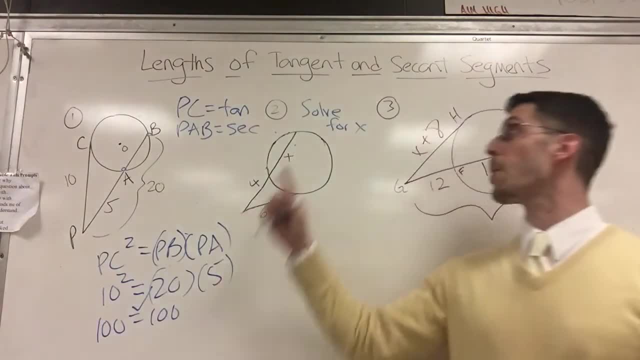 my math I proved my theory. Now we're going to do it when you actually have to solve. So if I have to solve for x, I'm going to be careful, because I've made mistakes in the past. Let me see here. Tangent is: 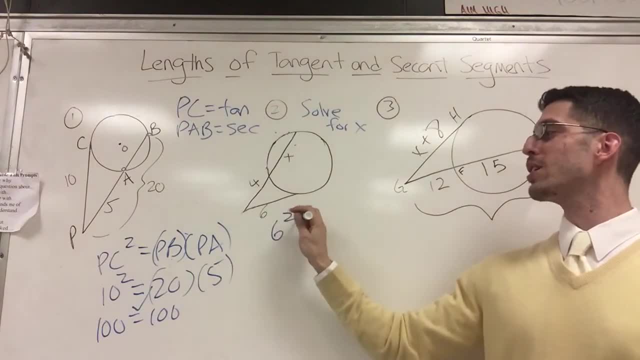 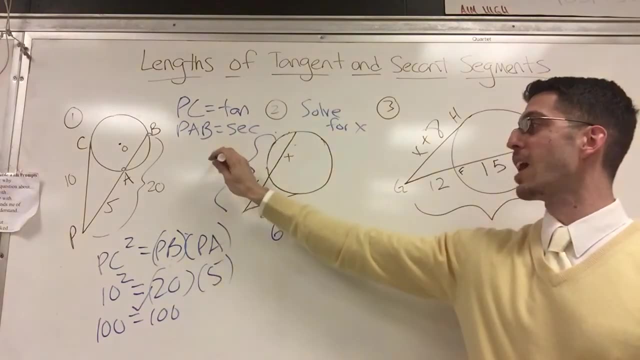 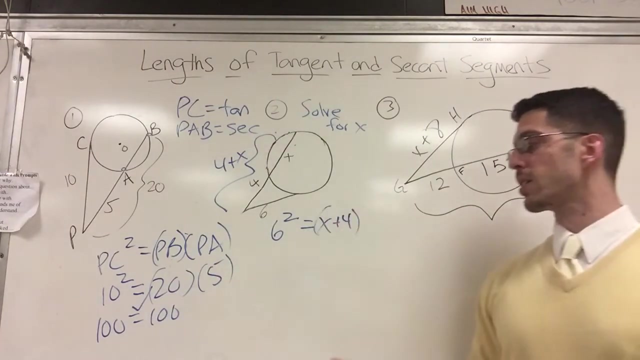 6. So 6 squared equals the entire thing. Is it 4?? No, Is it x? No, It's 4 plus x. The entire thing is 4 plus x, also known as x plus 4.. I prefer my x to go first, Not that there's anything wrong with. 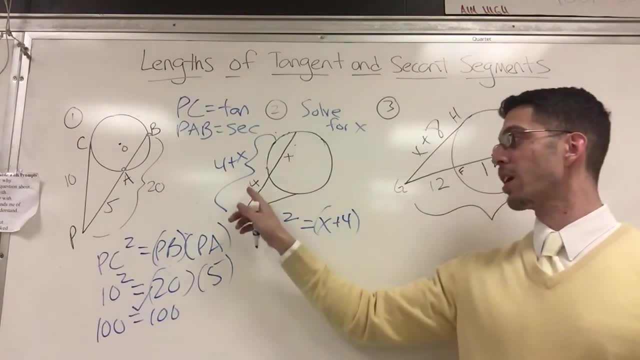 the other way. No one's going to win. I'm going to do it. I'm going to do it. I'm going to do it. I'm judging you. Okay Times, the external segment, which is 4. 4. All right, Now I want to solve for 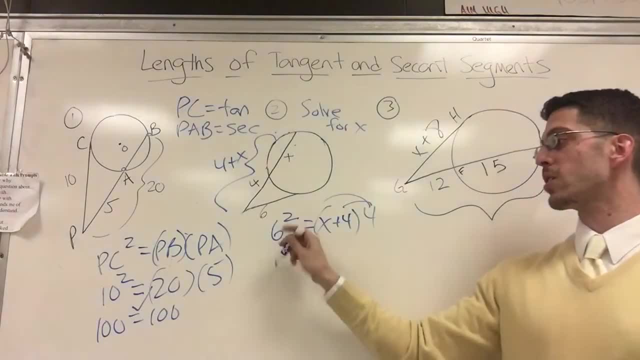 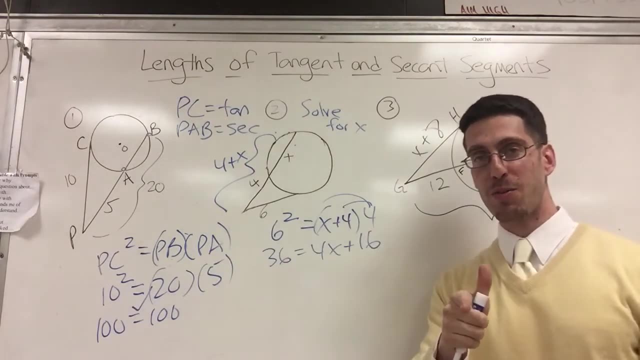 x. So I'm going to use my favorite property, which is a distributive property: 6 squared is 36 equals 4x plus 16.. Am I good? Everyone's following, Great Thanks. Now I want to get x alone. So since 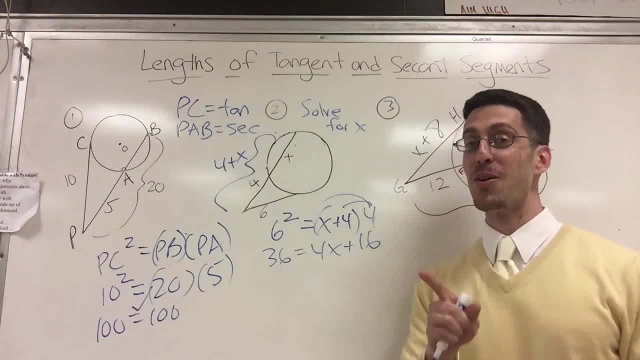 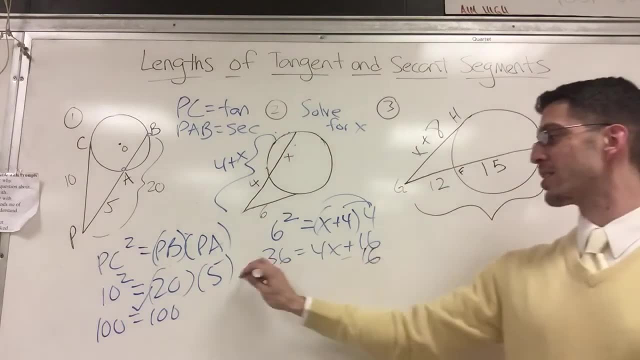 it's Sweater Fridays. I'm going to share a joke that a student told me. They told me: if you want to get x alone, buy it a drink, Okay. So I'm going to subtract 16 on both sides. 36 minus 16 is 20.. 20 equals 4x And, if I remember, 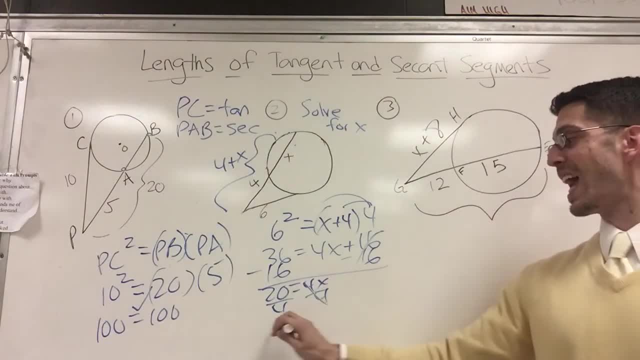 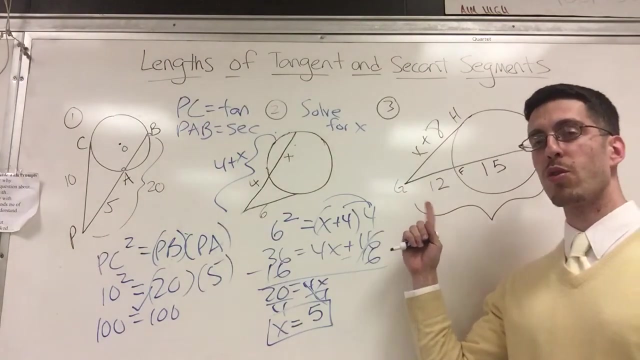 my math, then 20 divided by 4x equals, if you can see that, 5.. All right Now. thank you very much for your silent applause, you guys at home. One more: See if you can do this on your own, If you. 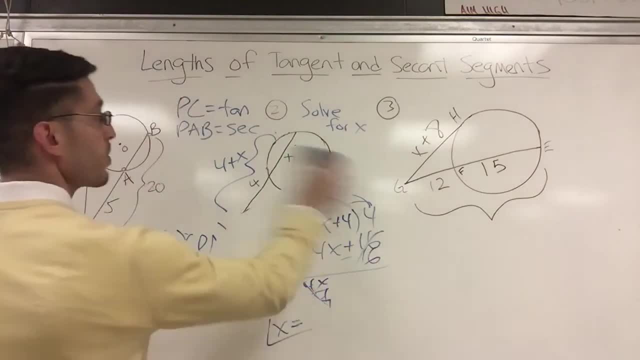 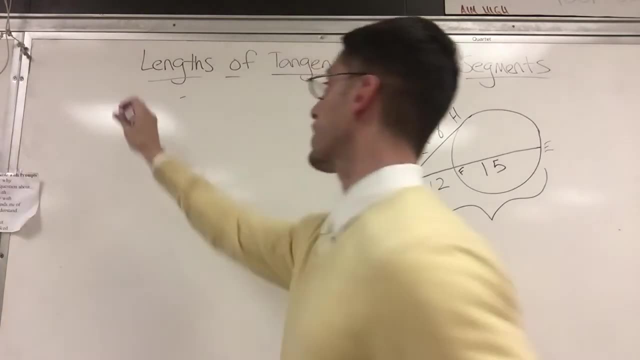 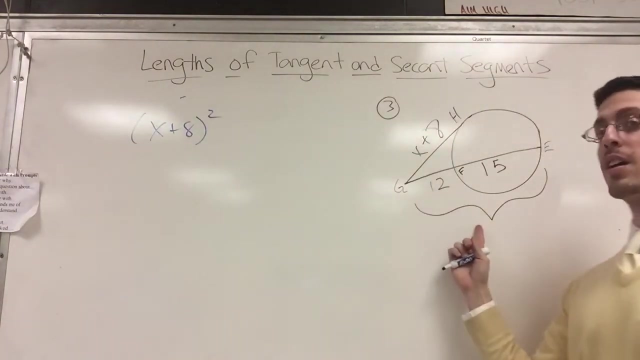 can't stick around. I'm going to do it for you. We got my external segment, which is x plus 8.. So I'm going to write x plus 8.. Oh, you're going to love this one. This brings back a lot of algebra. x plus 8, squared times the entire thing You're. 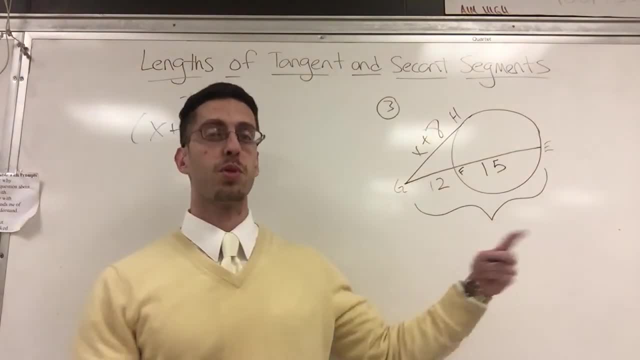 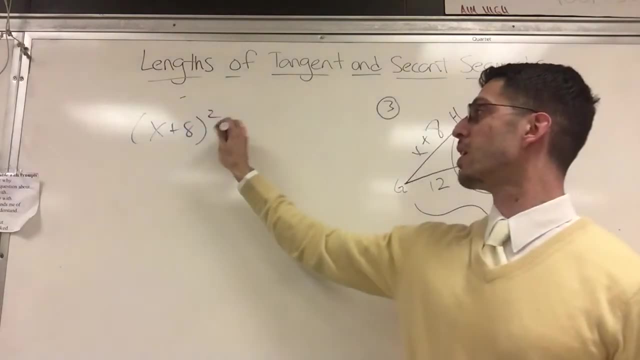 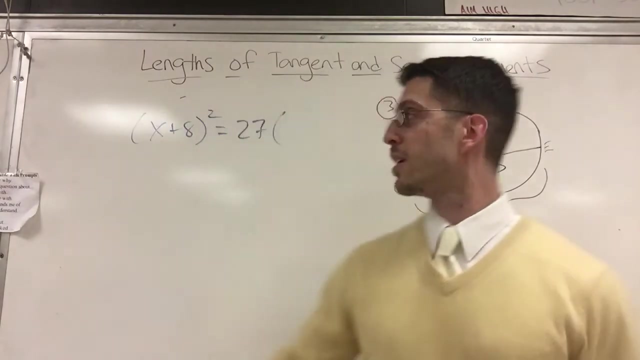 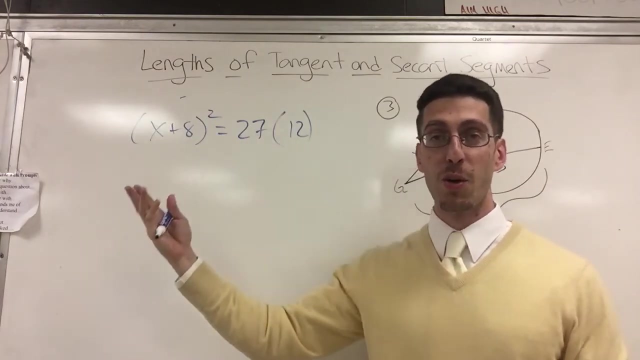 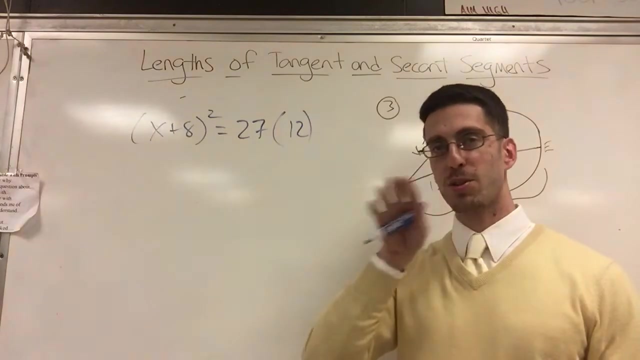 probably not going to see this wiggly-woggly on a test, but you should know it. So what is it? 12 and 15 together, That's 27.. So 27 is the entire thing, 27 times the outside, which is 12.. Okay, Here we go. Now that I set up my formula, I wish I had a calculator, or maybe someone in the audience could tell me what is 27 times 12.. And while I'm thinking about it, I'm going to do x plus 8 squared. Do you remember how to do this from algebra? Because there's no, I haven't done a video on it yet. Well, actually I have. If you could find it, I'm going to just step over here to my air calculator. I'm going to type 27 times 12.. 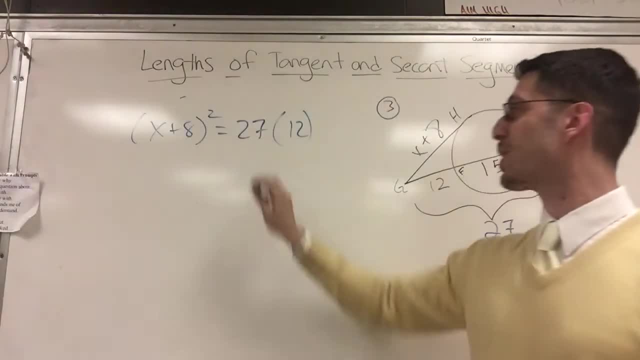 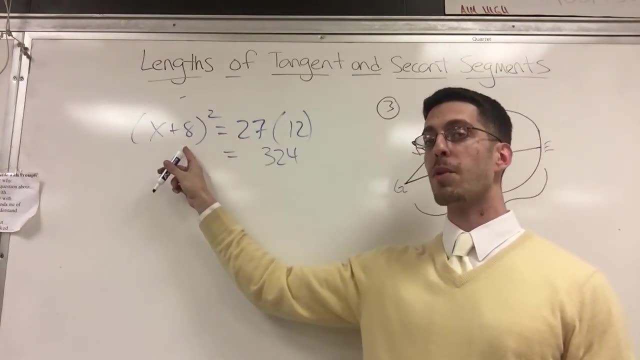 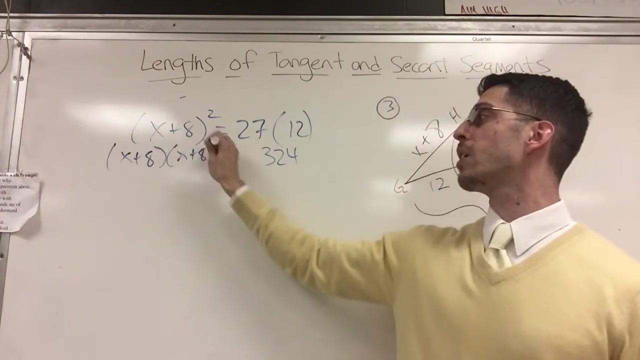 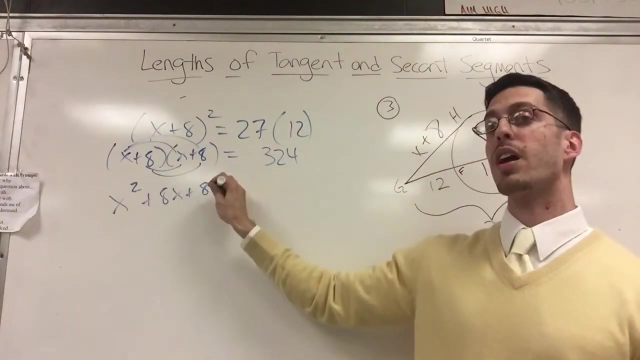 27 times 12.. 324.. Okay, The magic is happening. Beautiful air calculator, I love it. x plus 8 squared. I might have done a video a long time ago that said: how do you find the square of a binomial? You remember it? It's x plus 8 times itself. When I do that, I'm going to use something called FOIL, First outer, inner, last. That gives me x squared plus 8x, plus another 8x plus 64.. This is all review from algebra. 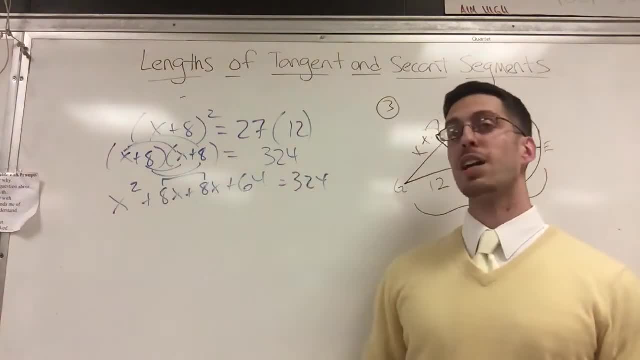 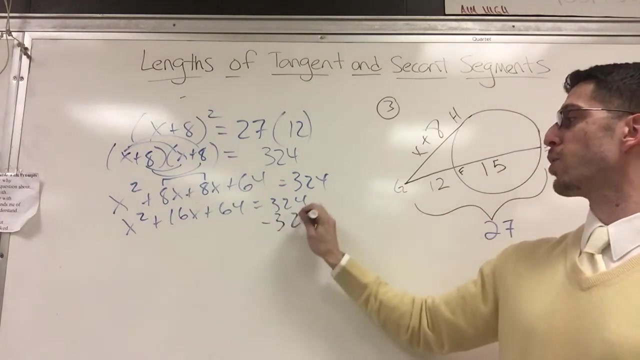 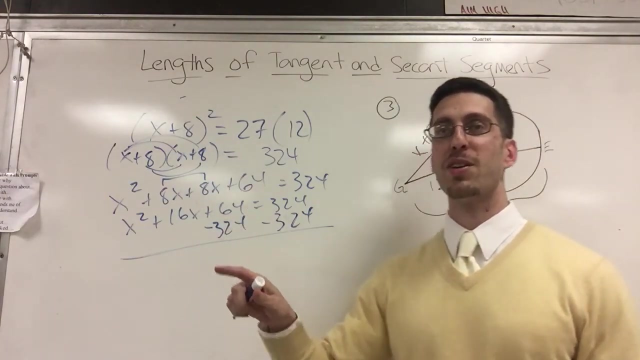 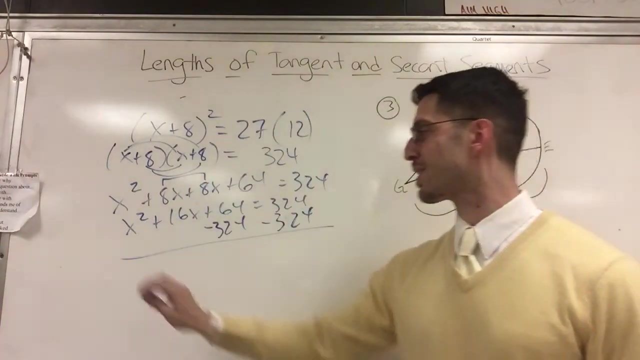 Equals 324.. Touchdown: Combine like terms: x squared plus 16x plus 64 equals 324.. Ah, here's something that I haven't done in a long time. This is called a quadratic equation. I want this side to equal 0.. So I'm going to subtract 324.. 324.. I'm doing 64 minus 324.. Let me go to my air calculator here And I'm going to guess that it's 260. for just to double check: Beep boop, beep boop, bop bop, Negative 260.. 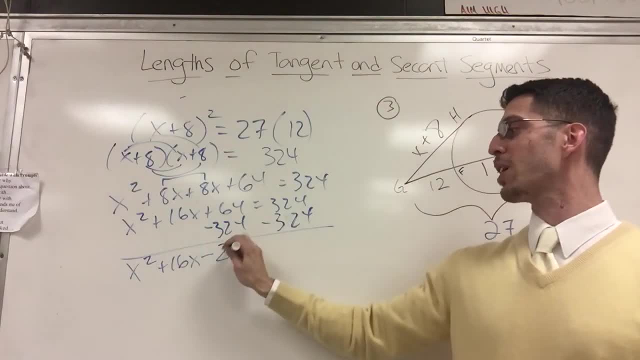 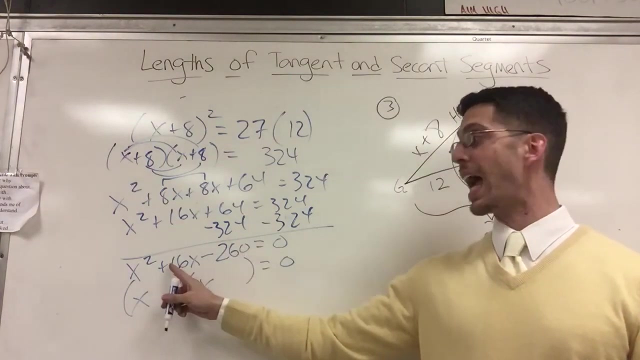 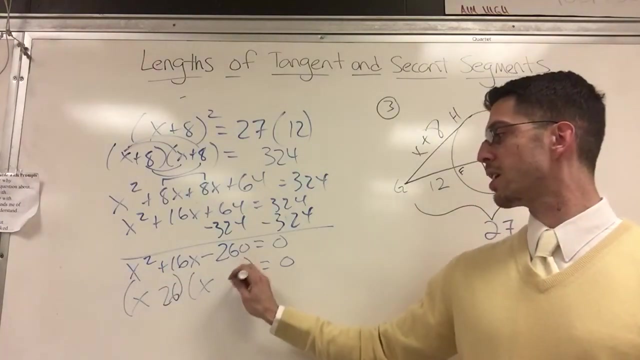 x squared plus 16x minus what did I just say? 260 equals 0.. Does this look familiar? Now you got to factor it: Boom, boom, boom equals 0.. I know an x and an x go here. I need numbers that multiply to 260 and add to 16.. I'm going to go with 26 and 10. And the bigger number gets the middle sign. So that's a plus.